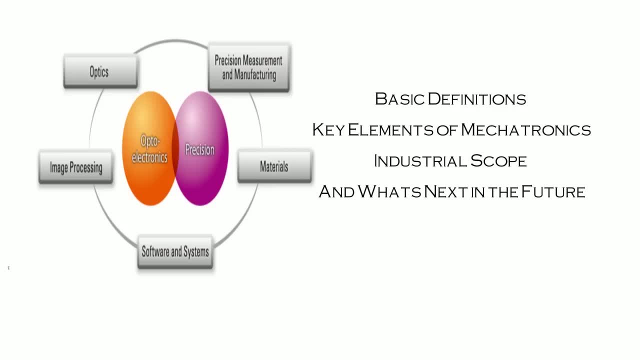 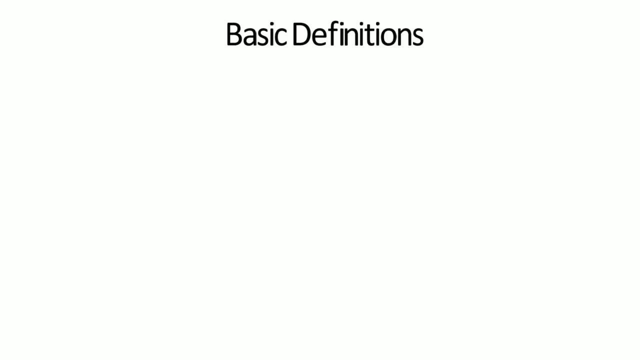 In this short video we will be discussing basic definitions, key elements of mechatronics, industrial scope and what's next. First, the definition of mechatronics has evolved since the original definition by the Yasukawa Electric Company. The word mechatronics is composed of mecha from mechanism and the tronics from electronics. 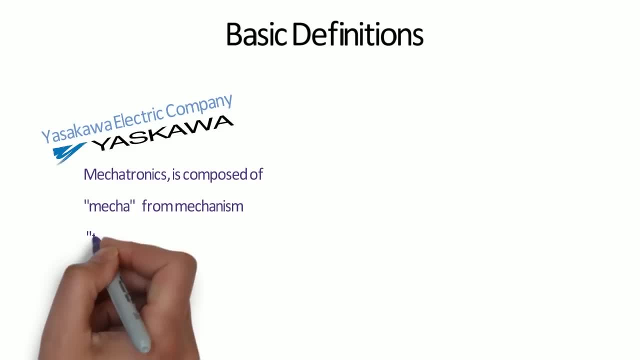 In other words, technologies and developed products will be incorporating electronics more and more into mechanisms, intimately and organically, and making it impossible to tell where one ends and the other begins. Another definition was presented by Hiroshima, Tomizuka and Furukawa. 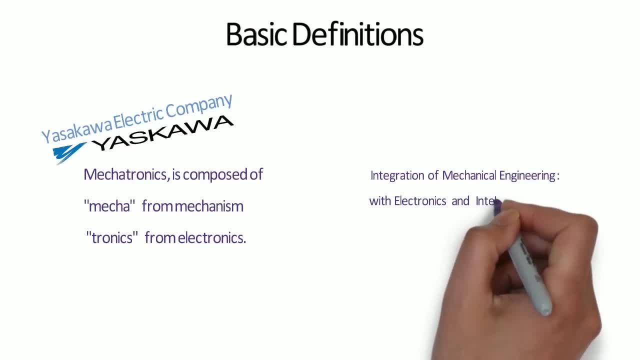 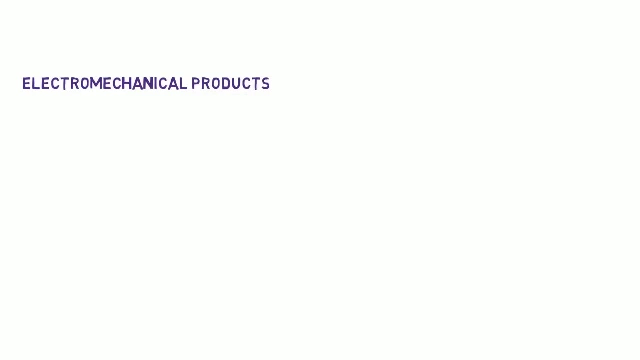 According to them, mechatronics is the synergistic integration of mechanical engineering with electronics and intelligent computer control in the design and manufacturing of industrial products and processes. Shetty and Koch in 1997 define mechatronics as methodology used for the optimal design of electromechanical products. 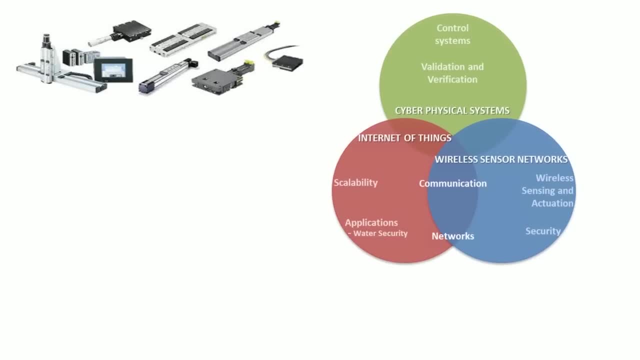 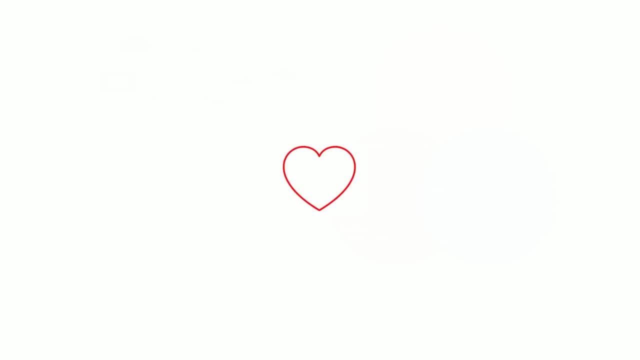 And Ausländer and Kempf suggested mechatronics as application of complex decision-making to the operation of physical systems, and W Bolton defined the mechatronics as not just a marriage of electrical and mechanical systems and is more than just a control system. 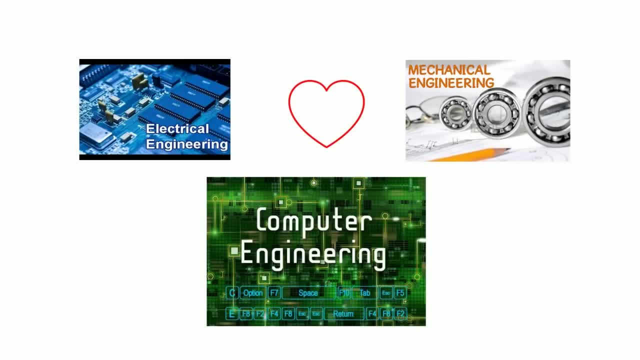 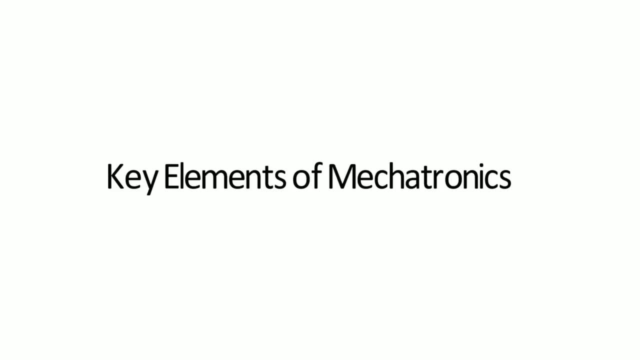 it is a complete integration of all of them. Now let's talk about the key elements of mechatronics. The study of mechatronics systems can be divided into the following areas of specialty: physical systems, modeling, sensors and actuators, signals and systems, computers and logic systems, software and data. 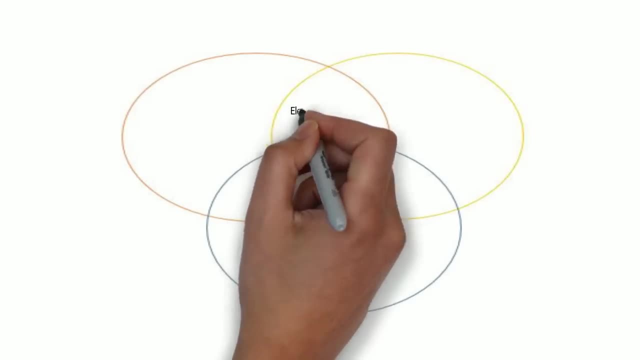 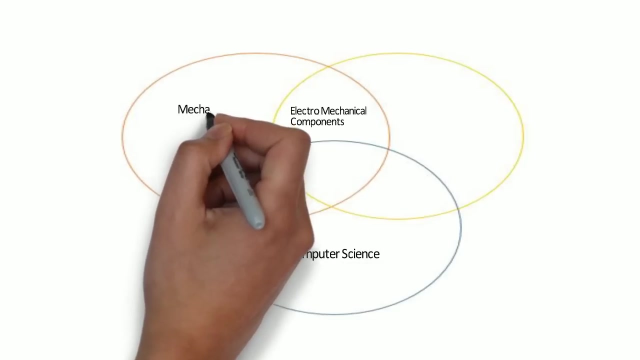 as well as the field of mechatronics. As the field of mechatronics continues to mature, the list of relevant topics associated with the area will most certainly expand and evolve. Mechatronic engineers can work with electronics and mechanical systems together and solve problems that cross discipline boundaries. 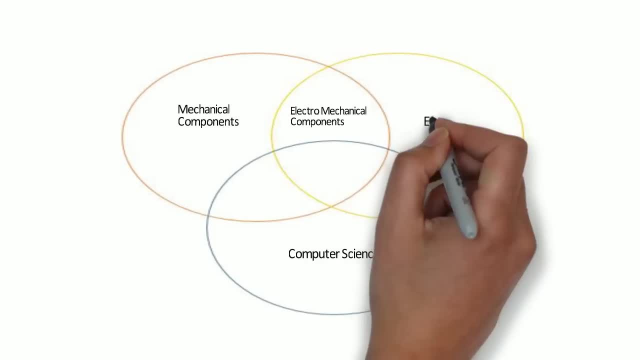 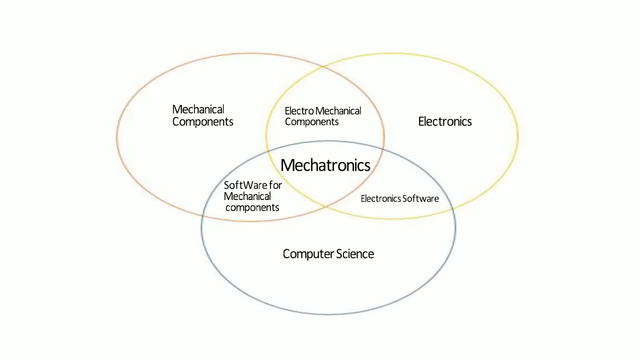 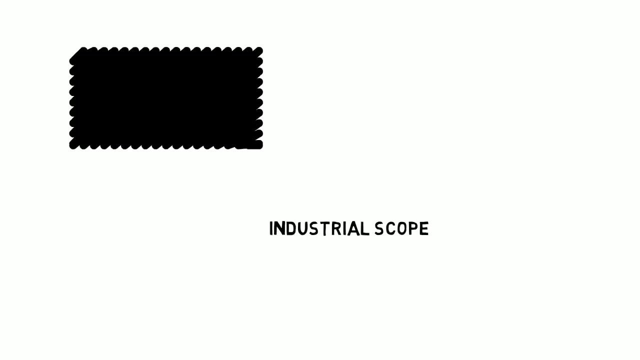 The list also includes Electromechanical components, Computer science, Mechanical components, Electronics, Electronics software, Software for mechanical components. Mechatronic engineering is the engineering discipline concerned with the research, design, implementation and maintenance of intelligent engineered products. Industrial scope of mechatronics: Some of the expert areas which mechatronics engineers can utilize: 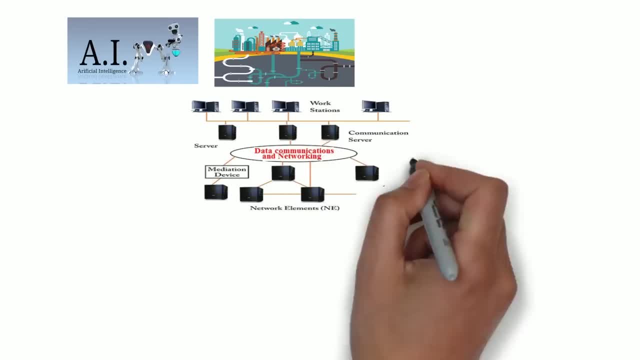 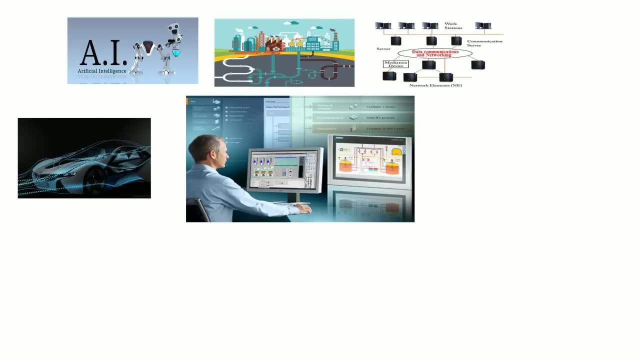 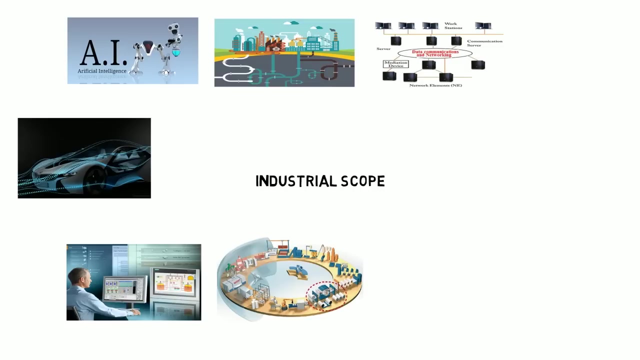 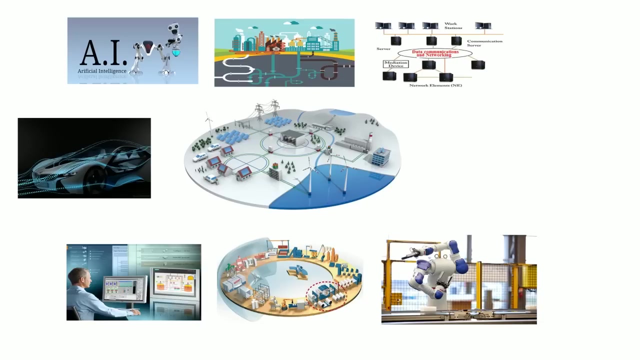 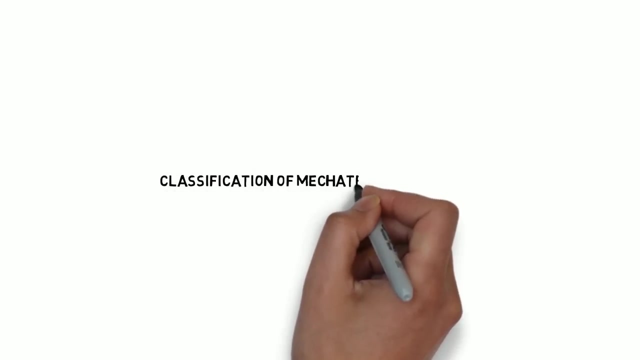 Artificial intelligence, control system, Data communications and networks, Dynamics of machines and mechanisms, Human machines, Machine interface, engineering and ergonomics, Industrial automation, process management, optimization and control, process, plant and manufacturing systems, Robotics, Smart infrastructure. In the late 1970s, the Japan Society for the Promotion of Machine Industry classified mechatronics products into four categories: 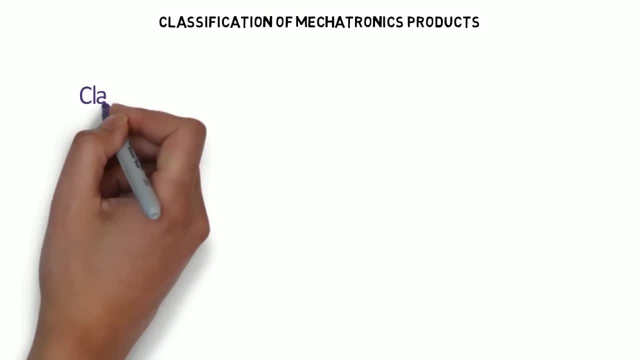 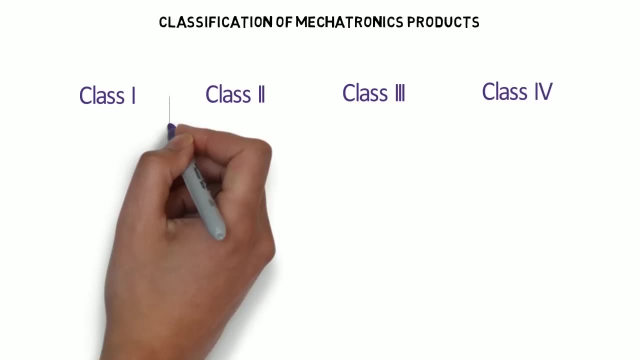 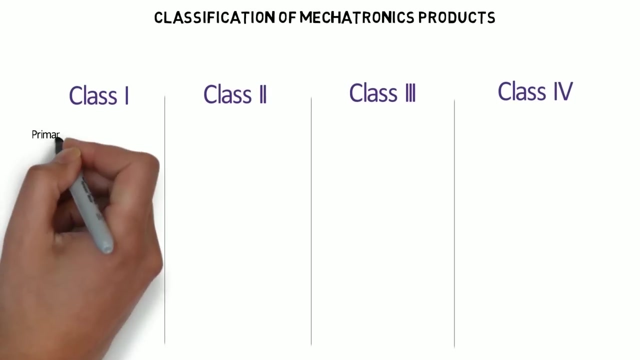 The enabling technologies for each mechatronic product class illustrate the progression of electromechanics, Electro-mechanical products in stride with developments in control theory, computation technologies and microprocessors. Class I products were enabled by servo technology, power electronics and control theory. 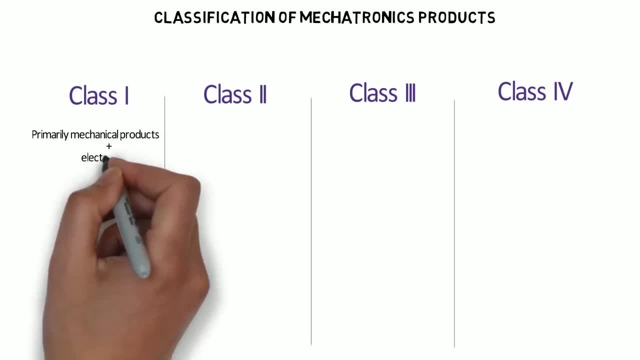 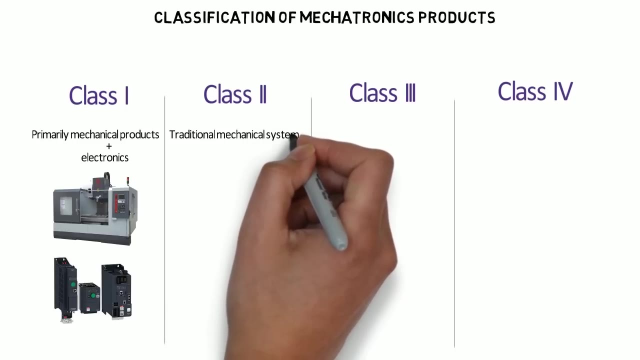 Primarily mechanical products with electronics incorporated to enhance functionality. Examples include numerically controlled machine tools and variable speed drives in manufacturing machines. Class II products were enabled by the availability of electronic components. Class III products were enabled by the availability of early computational and memory devices and custom circuit design capabilities. 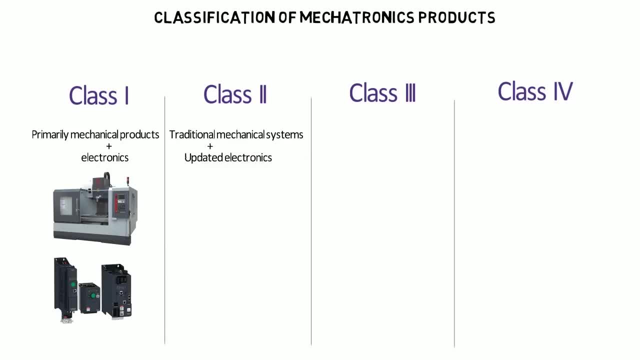 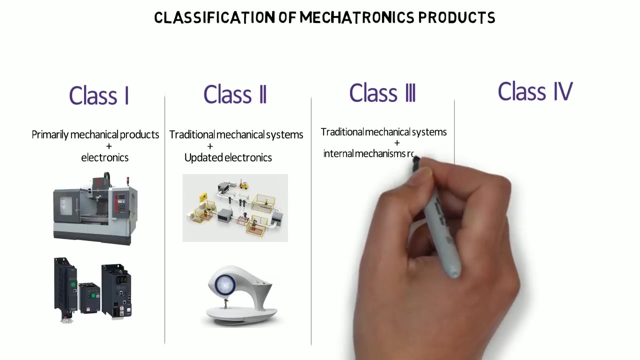 Traditional mechanical systems with significantly updated internal devices incorporating electronics. The external user interfaces are unaltered. Examples include the modern sewing machine and automated manufacturing systems. Class III products relied heavily on the microprocessor and integrated circuits to replace mechanical systems. Systems that retain the functionality of the traditional mechanical system, but the internal mechanisms are replaced by electronics. 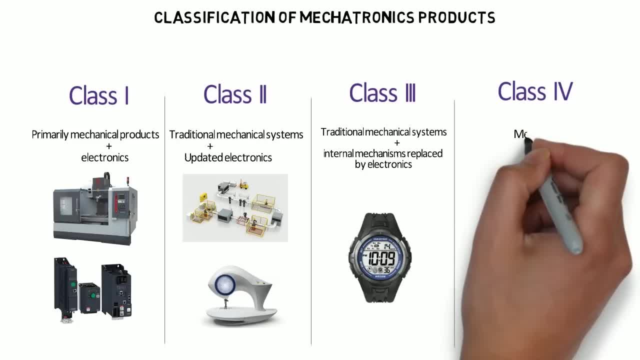 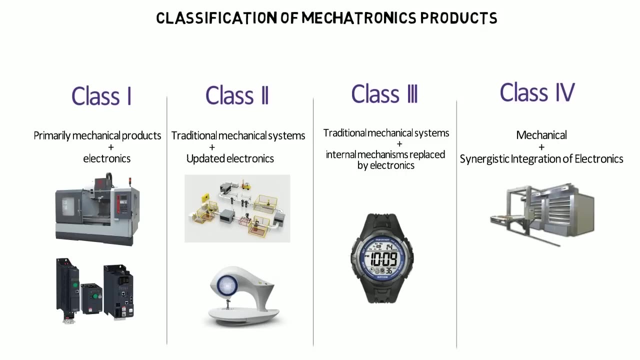 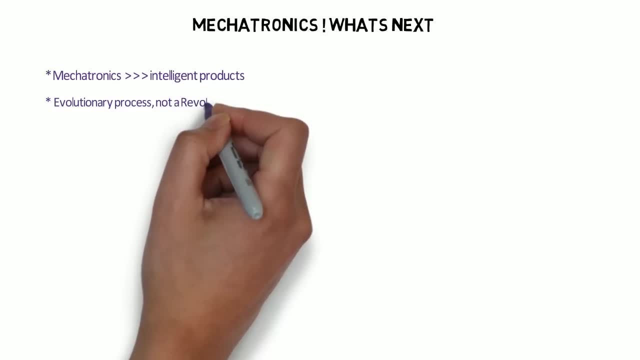 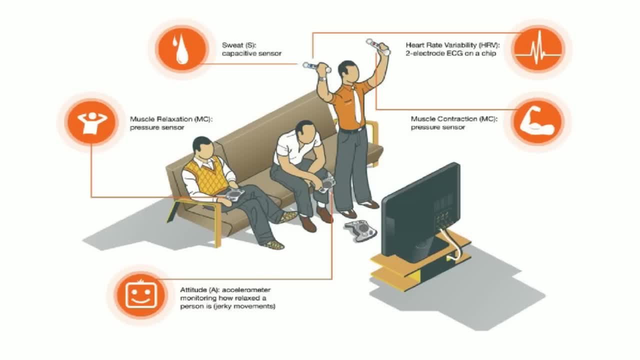 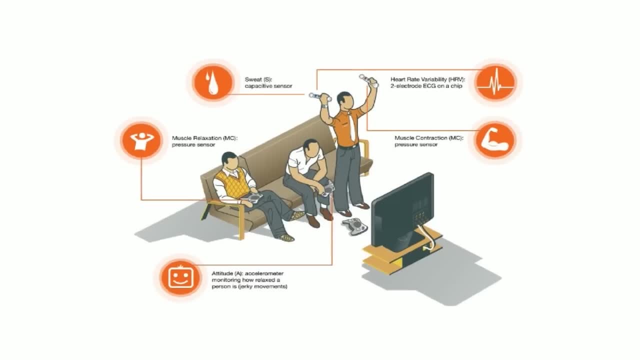 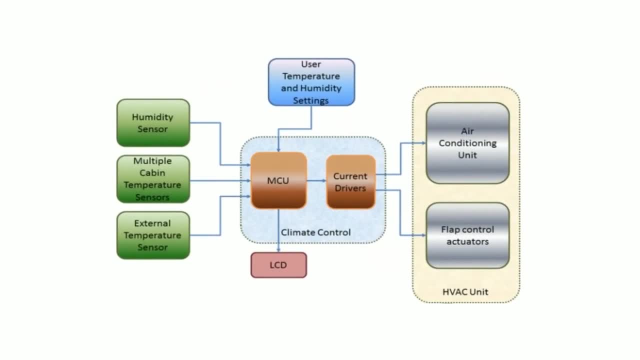 Already many mechatronic units possess rudimentary sensing abilities. Already many mechatronic units possess rudimentary sensing abilities. Already many mechatronic units possess rudimentary sensing abilities. For instance, modern air conditioning units are able to sense air temperature and humidity. 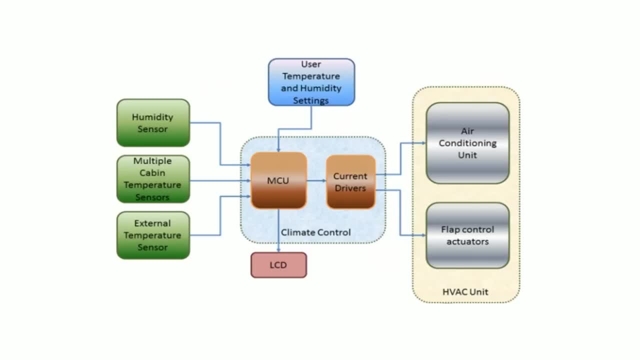 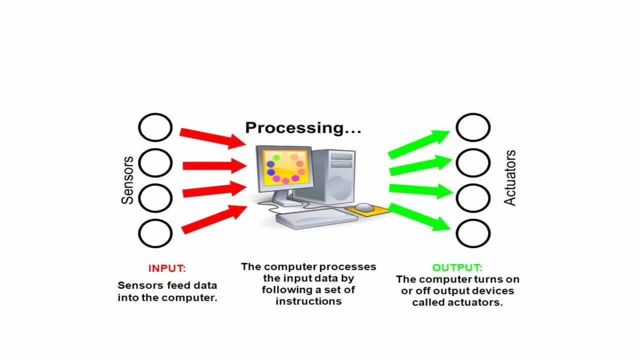 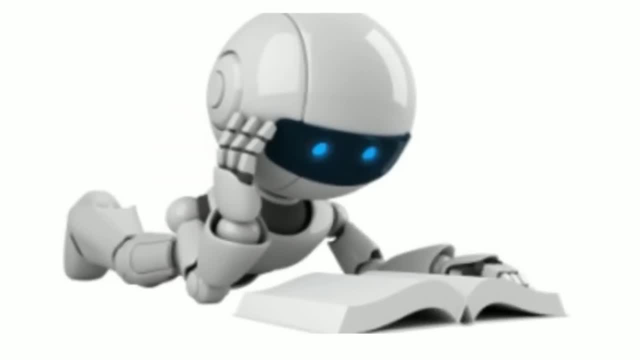 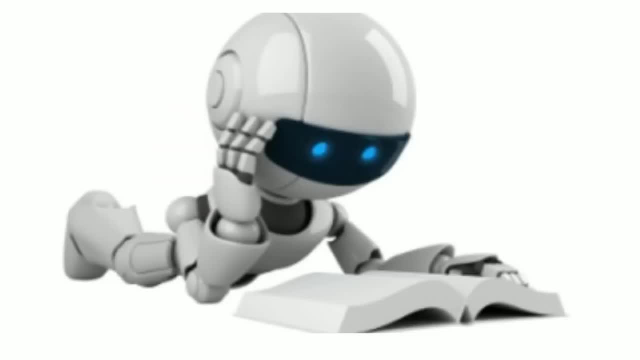